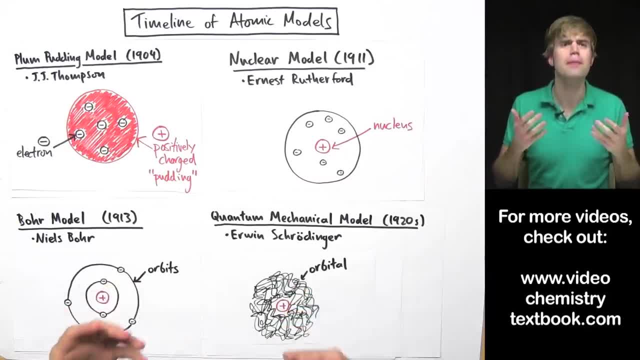 As scientists have done experiments and learned more and more about atoms, they've changed the way they think about atoms. So in this video, we're going to look at a timeline of the different ways that scientists have pictured or imagined atoms over the years. Now, the 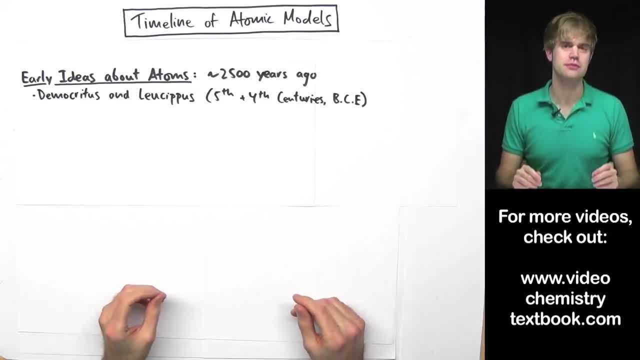 first people to really talk about the idea of atoms were the ancient Greek philosopher, Democritus and his teacher Leucippus. They lived about 2,500 years ago And, Democritus, he said something like this. He said: imagine you have an object like, say, a slice of bread. 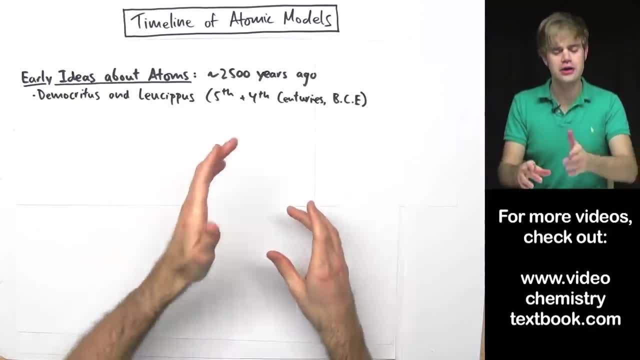 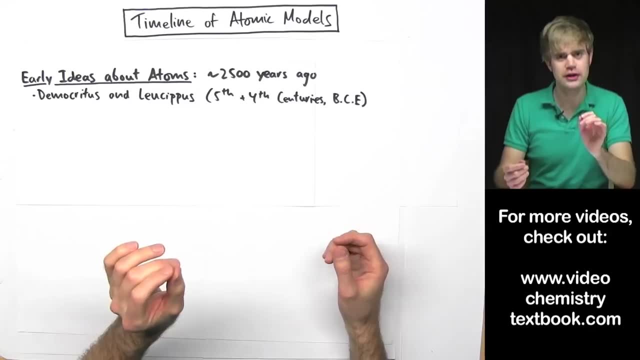 and you cut that in half, And then you take half of that and you cut it in half, And then you take half of that and you- well, you get the idea. Eventually, he said, you're going to come to something that you can't cut in half anymore. 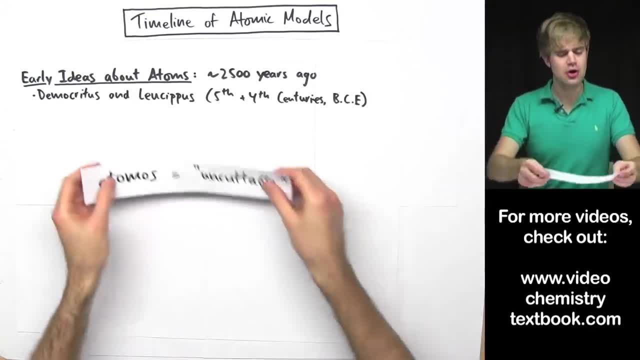 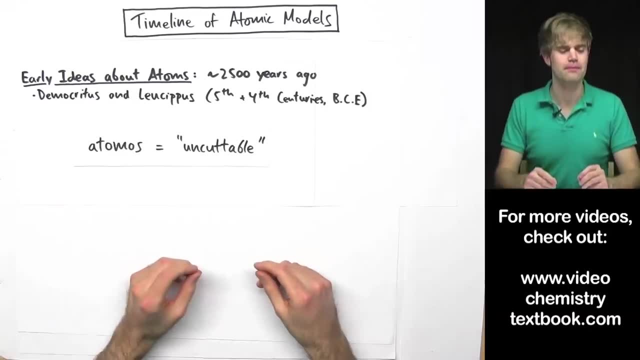 And then he said: you're going to come to something that you can't cut in half anymore. And he called these objects, he called them otomos, which means uncuttable, And it's where we get the word atom from. 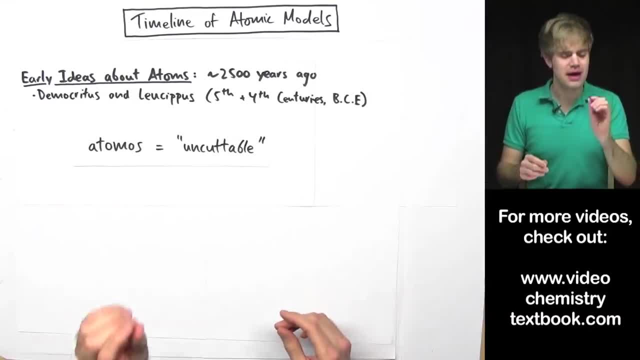 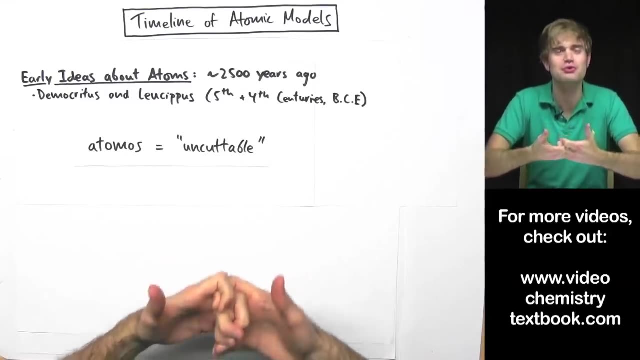 Democritus imagined that all matter, all stuff was made of these tiny, uncuttable particles, and he imagined that the atoms came in different sizes and different shapes. He imagined, for example, that iron atoms had hooks, which is how they could hold together so strongly and 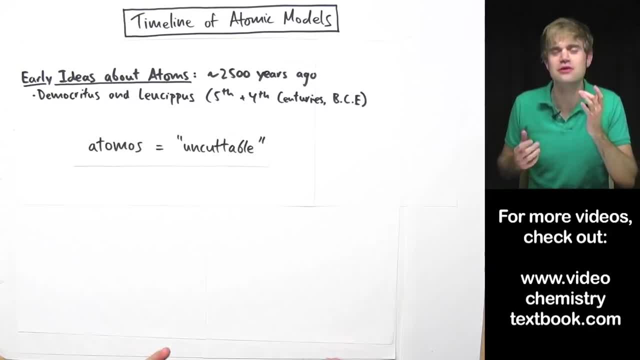 he thought that salt, which is a very important atom, has hooks, which is how they could hold together so strongly. and he thought that salt and iron had hooks, which is how they could hold together so strongly. and he thought that salt, Salt atoms- had spikes on them, because he felt that salt tasted sharp. 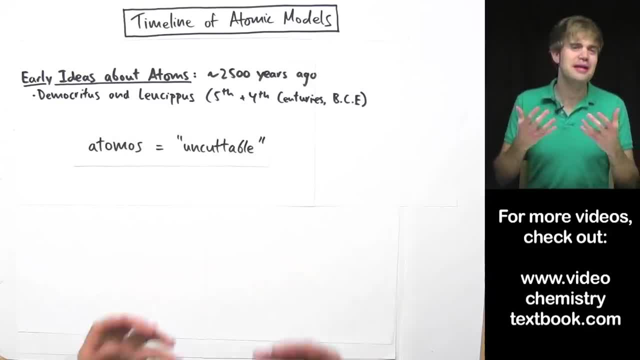 So Democritus was right, but people didn't really take to his ideas. Part of the reason was because, around the same time, the well-known philosopher Aristotle proposed his own idea of what matter was made of. He said that different things were made of different amounts of the elements: earth, water. 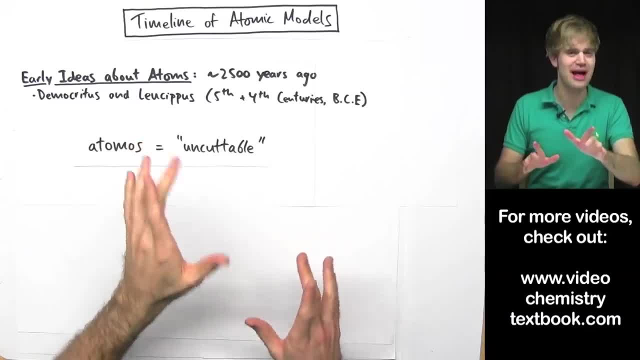 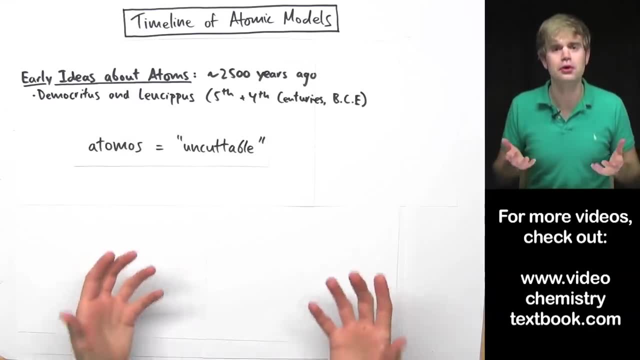 air, fire and ether. This is kind of like Captain Planet, if you're old enough to get that reference. And more people believed Aristotle, maybe just because he was so popular already. So Democritus and Leucippus, they were right all along. 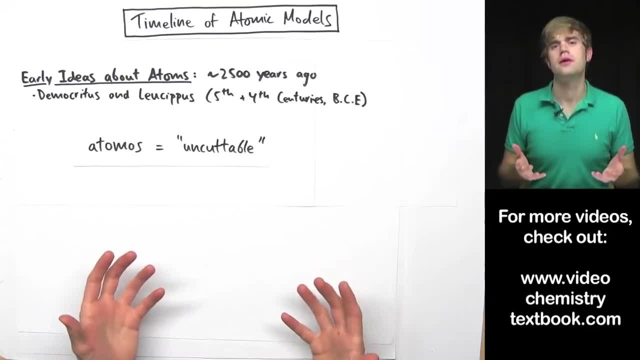 But here's the thing: they weren't scientists, They couldn't do experiments in the laboratory to prove that they were right. And because of this some people think that their idea it was just kind of a lucky guess. They couldn't actually prove what they thought. 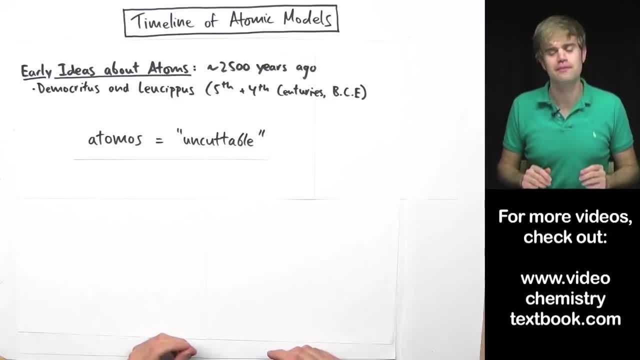 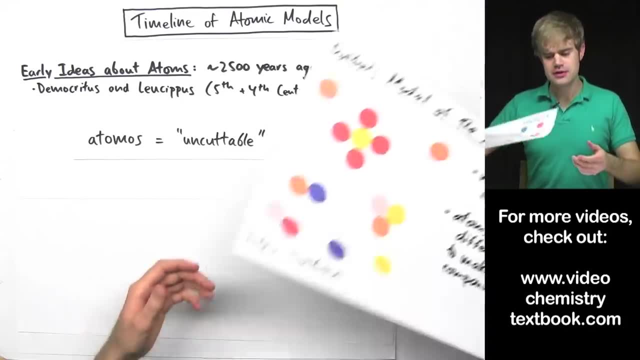 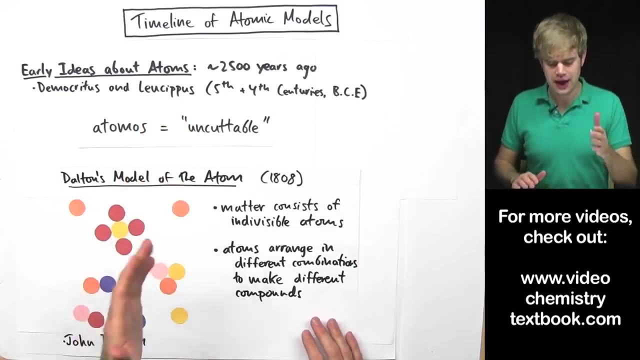 So you know, how can you tell whether it's right or wrong? Ideas about atoms remained that way for about 2,000 years until in 1808 the British chemist John Dalton came up with the first scientific experiments that showed that matter was made of tiny little particles. 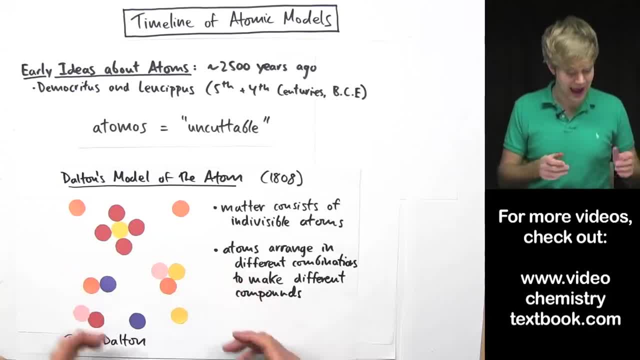 This is kind of how John Dalton pictured atoms. He imagined them sort of as tiny little balls that arranged in different combinations to make different things, And he imagined that these atoms were indivisible. You couldn't cut them into smaller pieces Now. at first nobody believed Dalton. 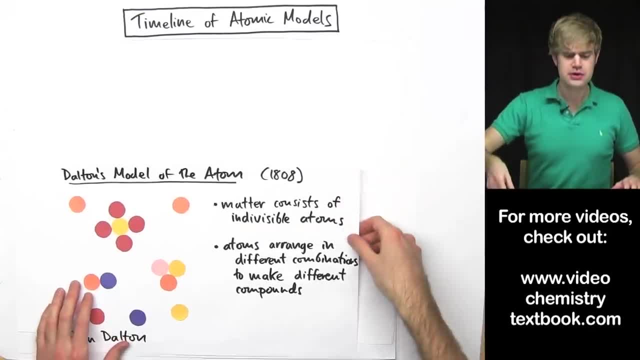 But over the course of the 18th century the British chemist John Dalton came up with a scientific experiment that showed that atoms were made of tiny little particles, And in the course of the 1800s more and more scientists did begin to believe what he had. 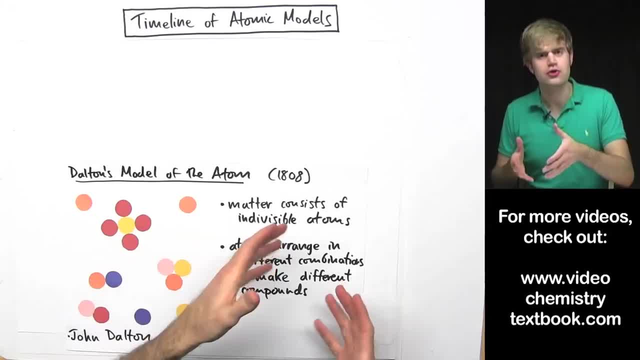 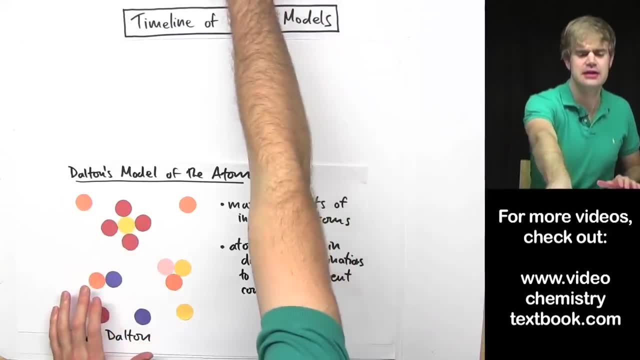 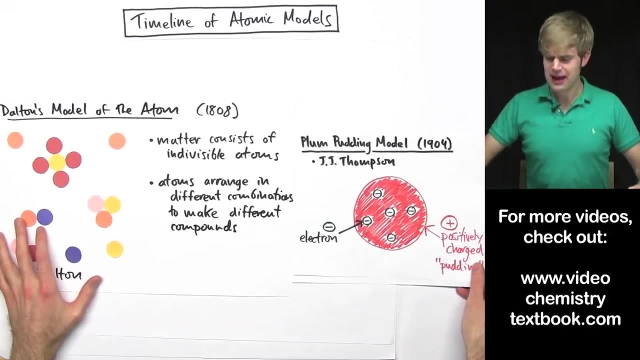 to say. But then in the 1900s- the early 1900s- people's idea about atoms started to change. One of the key things that caused this change was that in the late 1800s, JJ Thomson discovered that atoms have electrons. 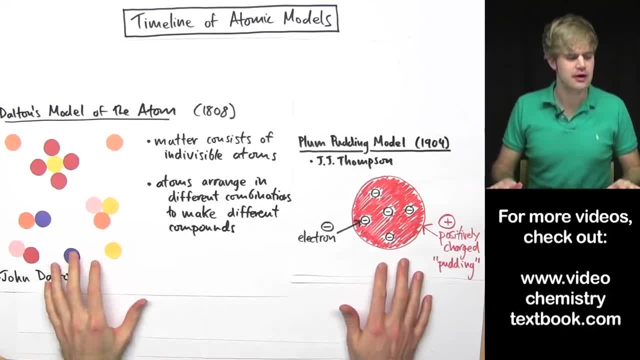 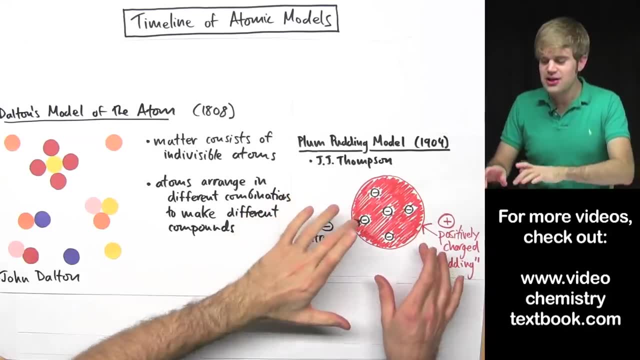 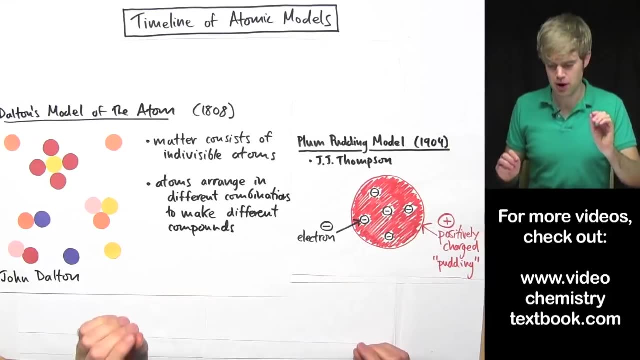 And he discovered that electrons are much, much smaller, Smaller than atoms. So while Dalton thought that atoms were tiny and indivisible, JJ Thomson said: no, no, they're not indivisible, because they're made up of electrons which are much smaller. 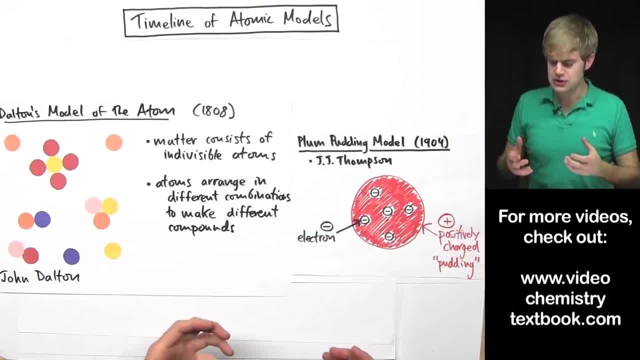 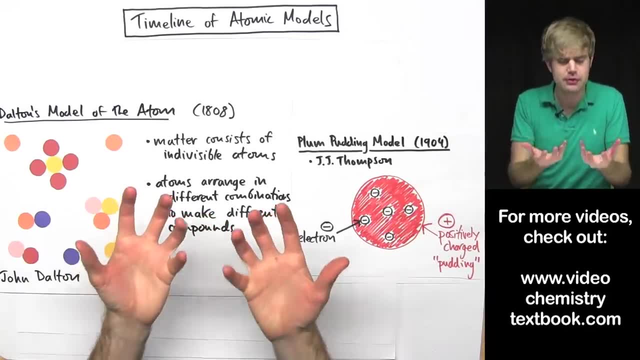 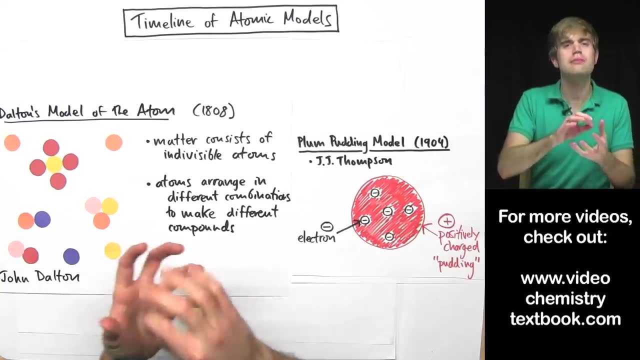 So JJ Thomson pictured the atom as sort of like a blueberry muffin. He called this the plum pudding model. JJ Thomson imagined that if you took an atom and split it open, you'd see tiny electrons stuck throughout the inside of it, just the way blueberries are stuck in the dough of. 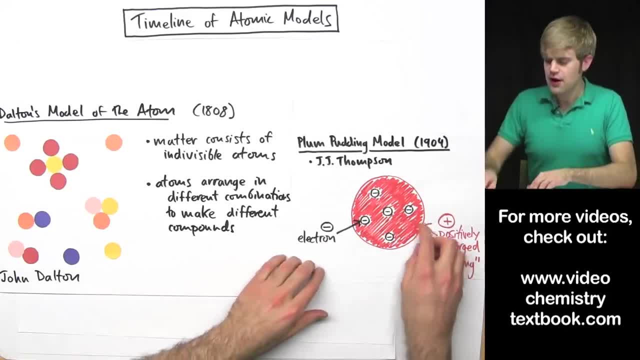 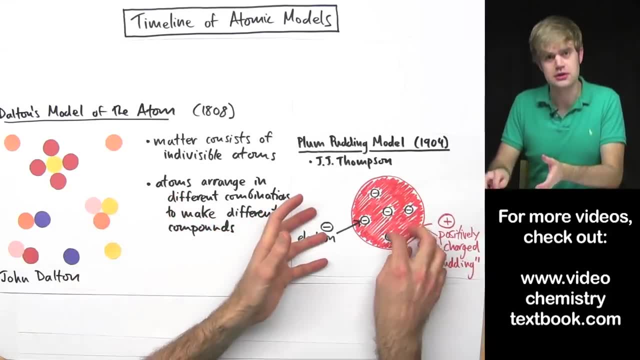 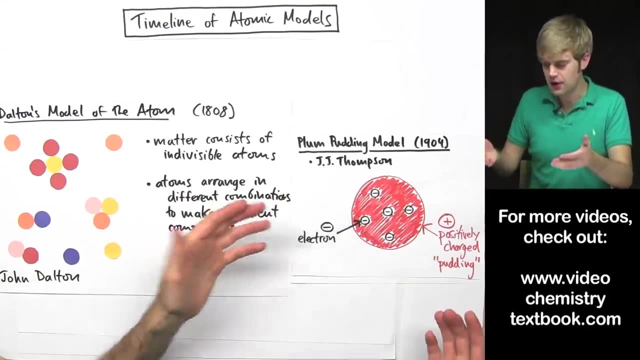 a blueberry muffin And Thomson thought that what's the dough in a blueberry muffin? That it was like a positively charged substance. So you had negative electrons stuck in like a positively charged dough And together the positive and negative charge balanced. 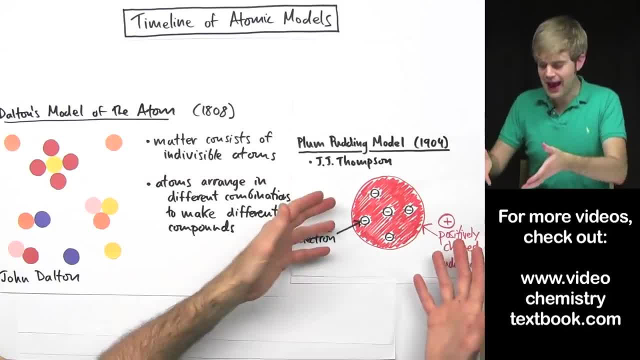 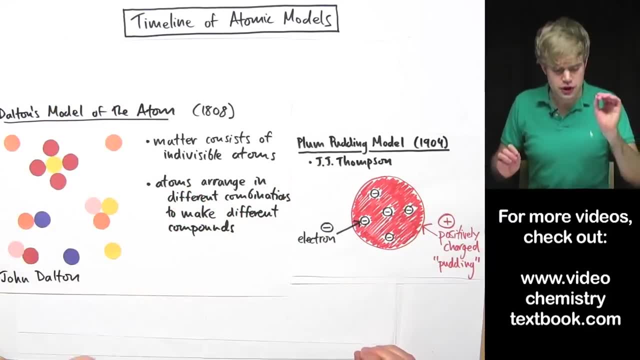 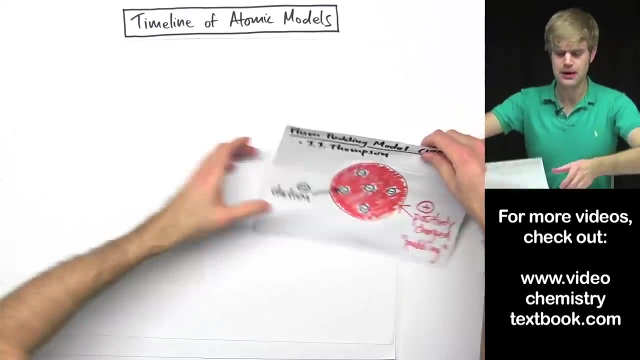 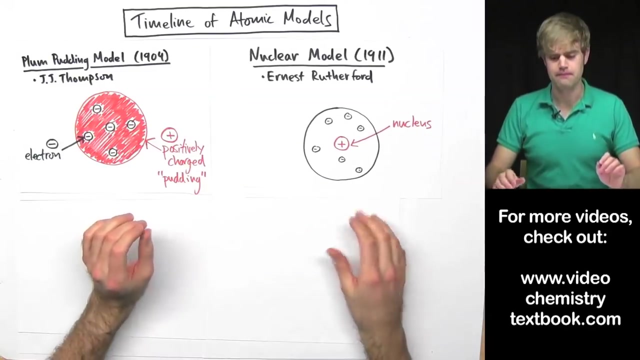 The two things balanced. They balanced each other out so that the atom was electrically neutral. But the big change from Dalton's model to Thomson's model was showing that atoms weren't actually indivisible, that they were made of even smaller things. Now, not too much longer. in the gold foil experiment Ernest Rutherford discovered that. 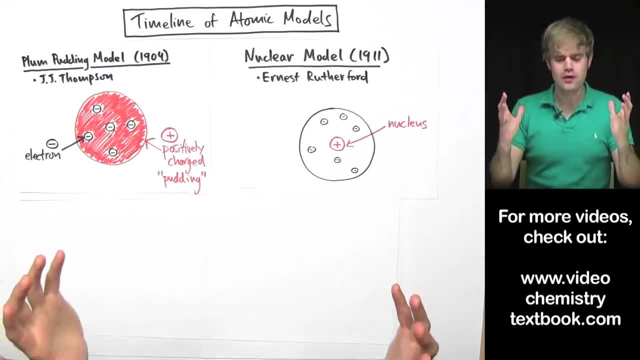 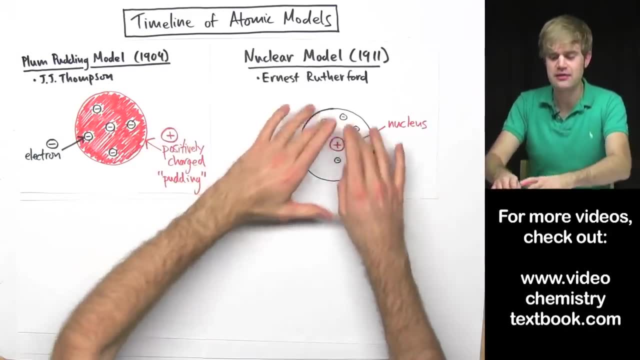 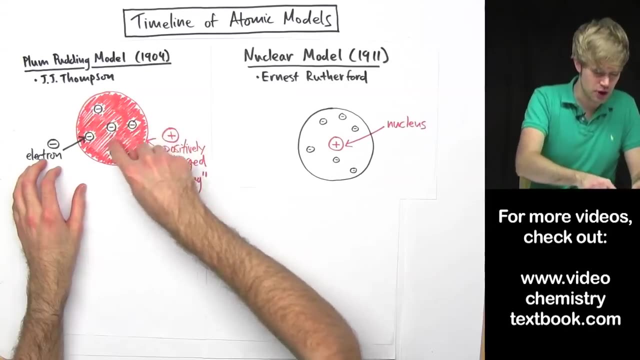 atoms had a nucleus. All the positive charge in an atom was concentrated right in its center and that besides that and the electrons, atoms were pretty much empty space. So JJ Thomson thought the positive charge was all distributed throughout like dough in a muffin. 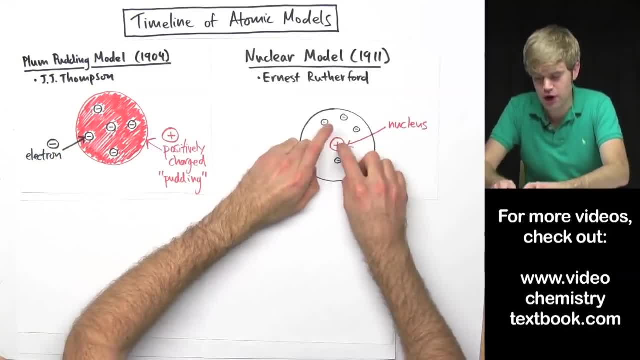 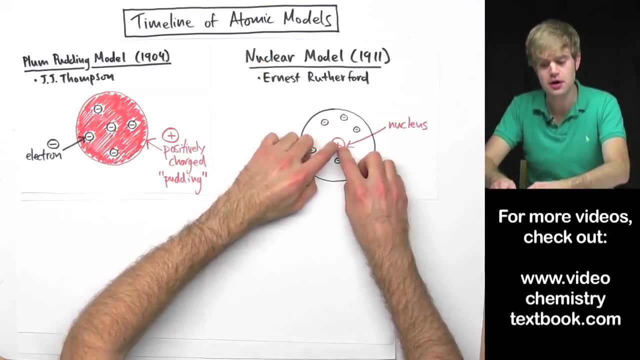 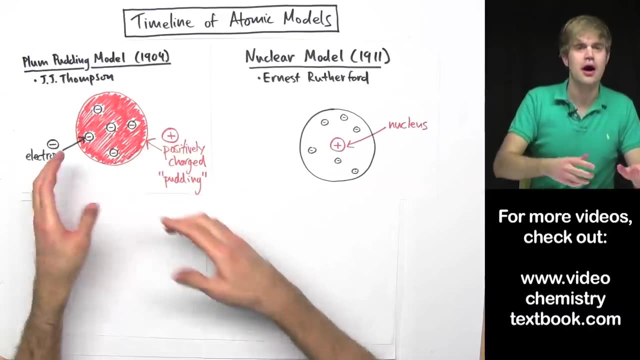 but Rutherford showed that all this positive stuff was concentrated right here in the center, And this is what we call the nuclear model of the atom, because it has a nucleus. Sometimes people call this the nuclear model, The Rutherford model. Now, so far we've been talking a lot about the positive charge and the nucleus of an 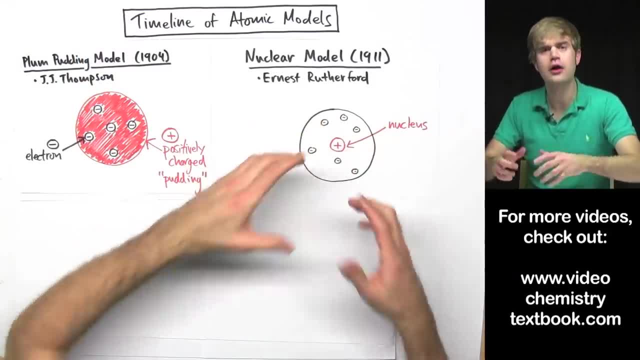 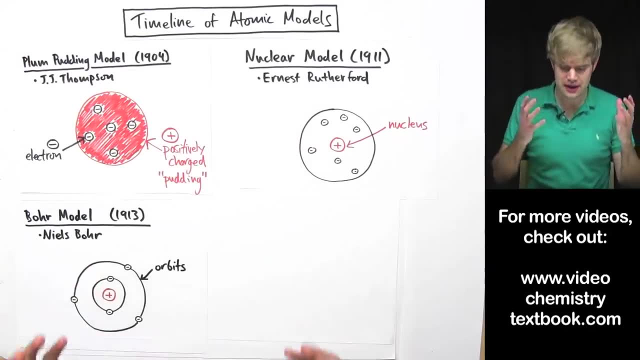 atom. But we haven't talked too much about what's actually going on with these electrons in the atom. And in 1913, the physicist Niels Bohr came up with his model of the atom. He reasoned that there is a nucleus in the middle, just like Rutherford had, but that 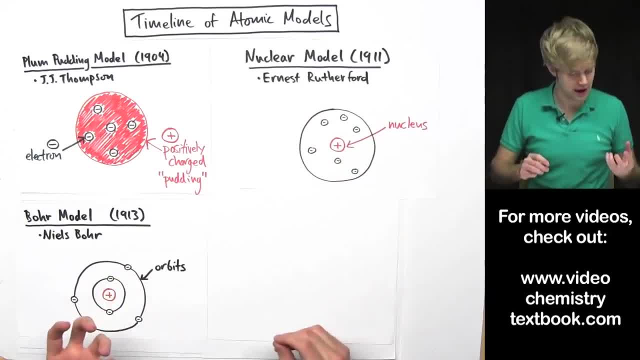 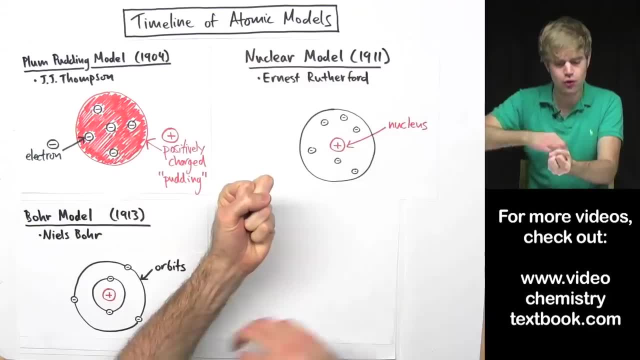 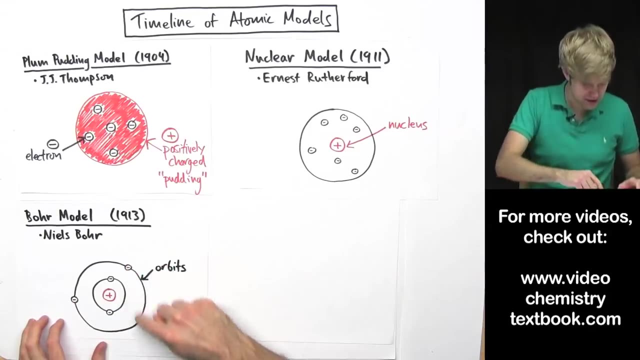 electrons, instead of just sort of being randomly distributed throughout the atom, brought a lot of energy, And Bohr said that the electrons were sort of like planets around a sun, that they were spinning around the nucleus in circular orbits. So here are a picture of some of the electrons and here are the orbits. 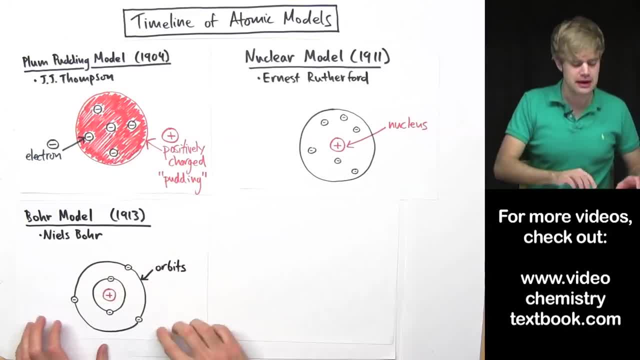 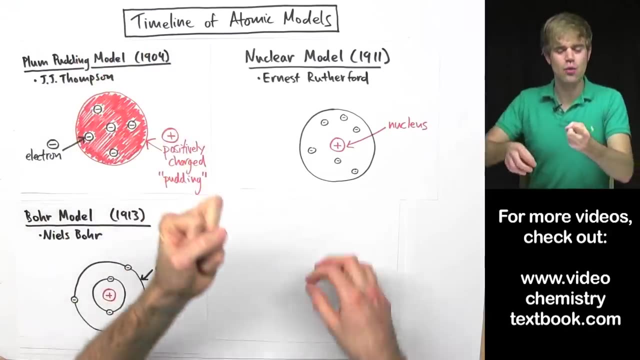 Imagine that they're spinning around the nucleus in these circles. Alright, now people thought Bohr's idea for the electrons made a lot of sense at first, But then, in the 1920s, Additional experiments showed that it wasn't exactly the way electrons really move. 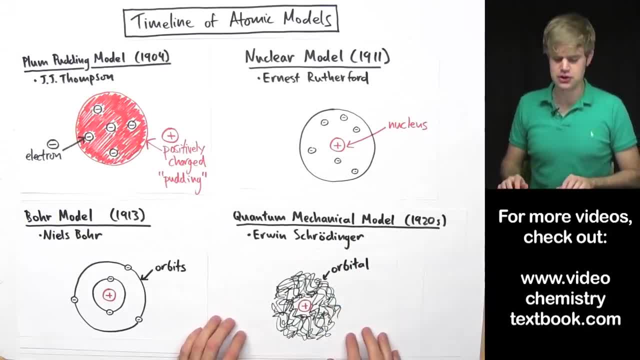 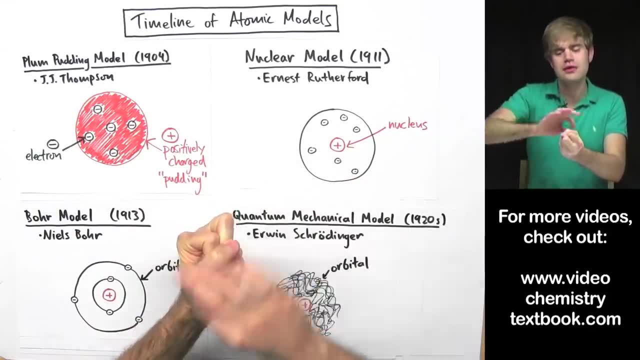 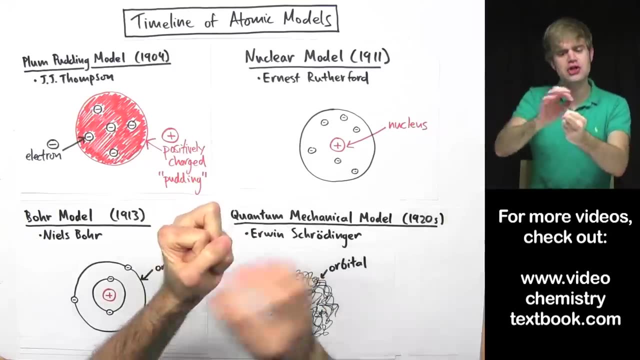 And a variety of physicists, particularly the physicist Erwin Schrödinger, showed that electrons weren't really spinning in orbits, but it's more like they were hyperactive flies, and they were buzzing around the atom, sketching out different shapes. 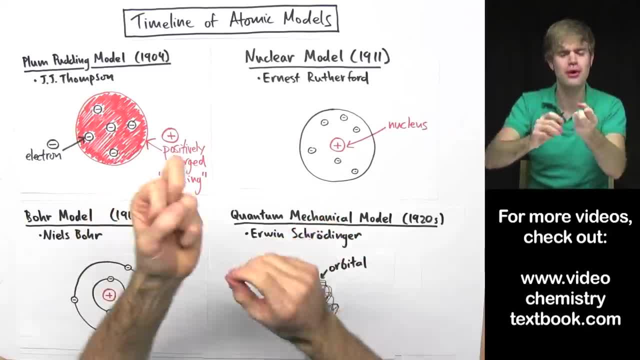 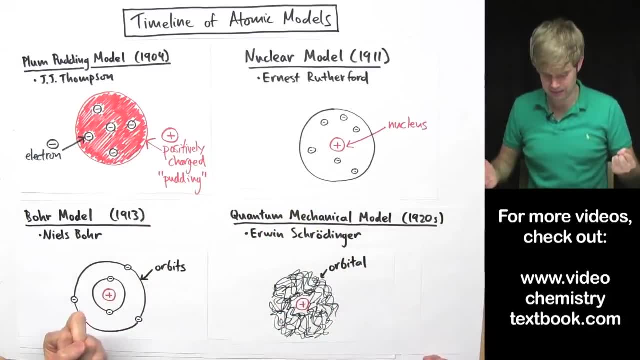 It's kind of It's like time-lapse photography on a hyperactive fly and you saw that over a long period of time it sketched out a particular design And whereas Bohr called these circular paths, he called them orbits, Schrödinger called 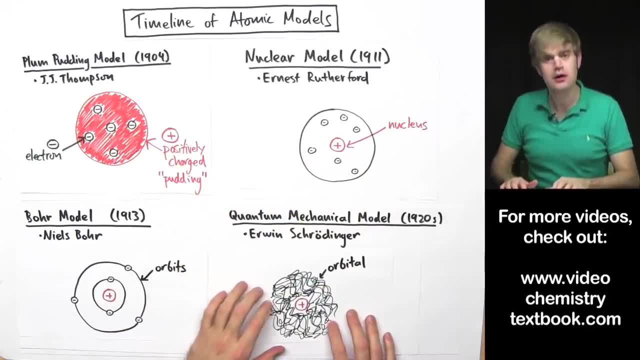 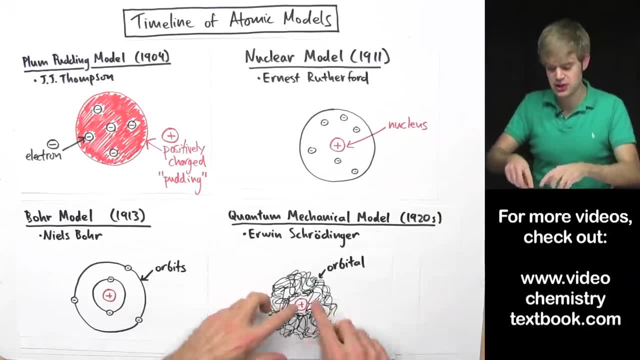 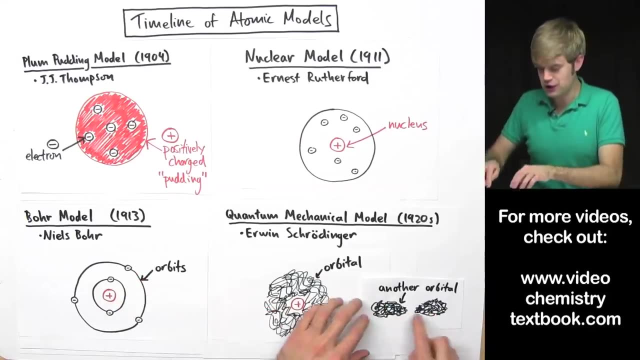 the hyperactive sketch-out shapes. he called them orbitals. Here's a circular orbital too, But electrons didn't only make circles. This is actually a sphere, because it's a circle in three dimensions. Here is another shape, another type of orbital that electrons could also make. 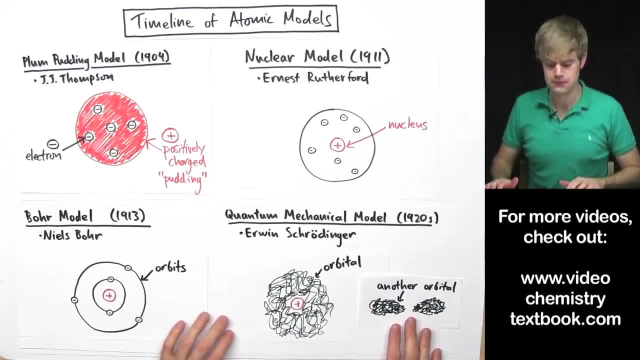 Looks like this sort of two teardrops next to each other. So in the quantum mechanical model, electrons don't orbit the nucleus. They buzz around the atom, sketching out different shapes. Now let's focus on the nucleus here. Over the same amount of time and a little bit later, scientists were trying to figure. 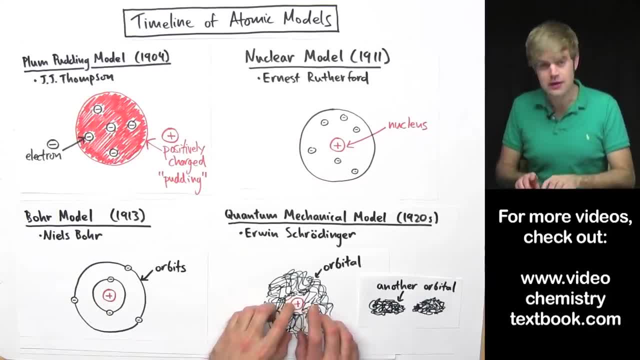 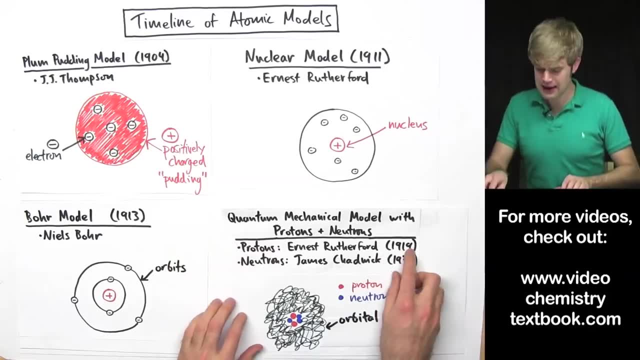 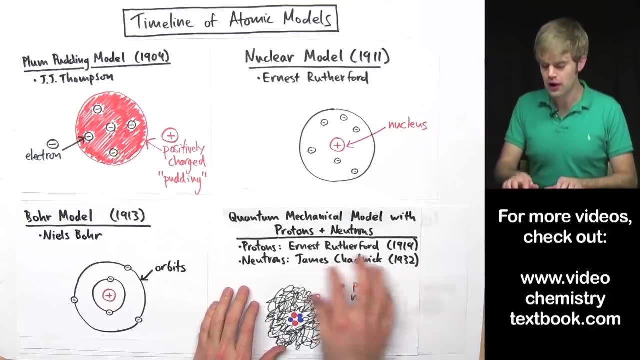 out the two subatomic particles that make up the nucleus. So we can refine this picture a little bit more. In 1919, Ernest Rutherford discovered protons. There they are. And then in 1932, James Chadwick discovered neutrons. 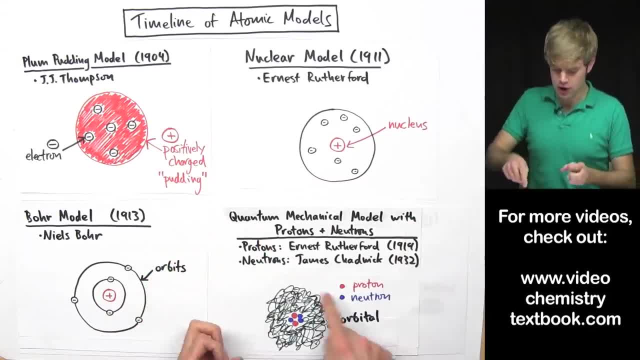 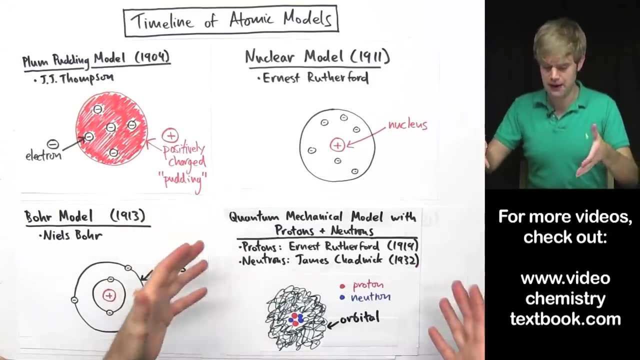 So the really correct view of the quantum mechanical model shows the orbitals being sketched out by the electrons, But then also shows the subatomic particles. The subatomic particles protons and neutrons here in the nucleus. Now this is pretty much how we think about atoms today.